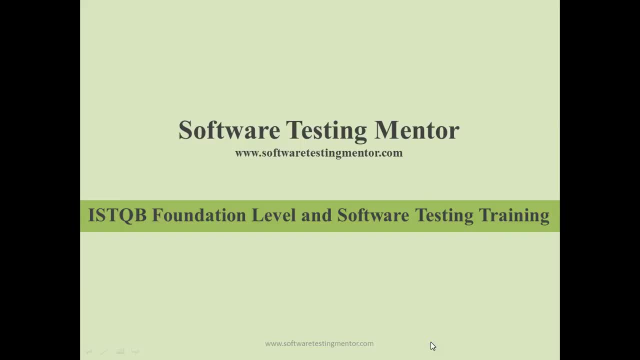 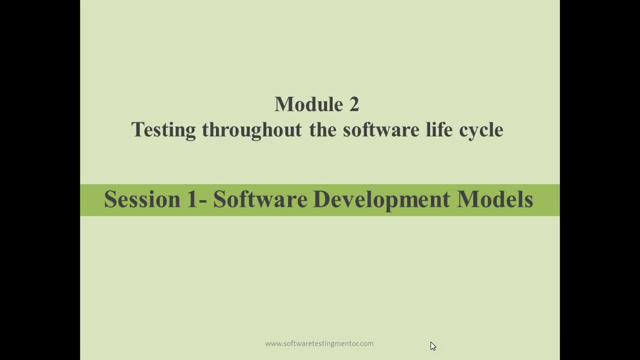 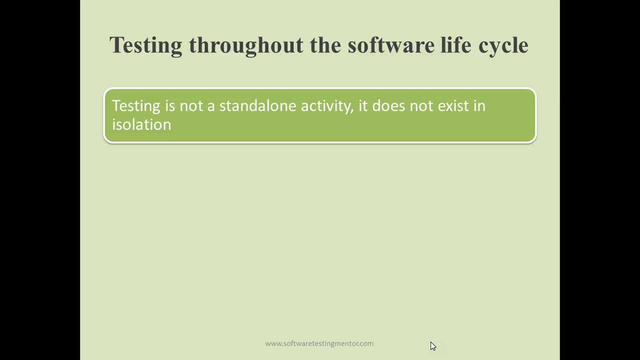 Hello everyone, Welcome to session 1 of module 2, software development models. In this session I will cover different software development models and how testing is done throughout the software lifecycle. So testing is not a standalone activity. It does not exist in isolation Testing. 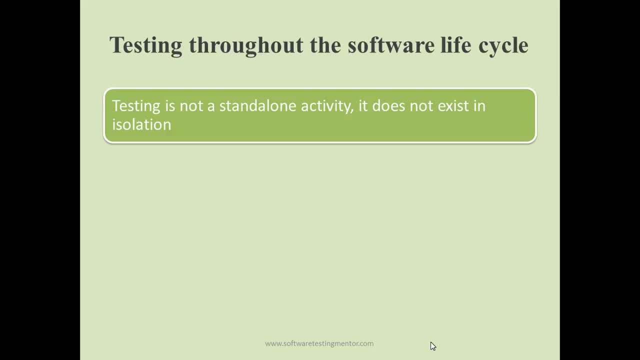 is dependent on what type of software development lifecycle is being followed. So, depending on the development lifecycle, testing fits in that lifecycle and testing is done in every phase of the development lifecycle. so if you are following waterfall development methodology, testing has its own place in that software development model. If you are following 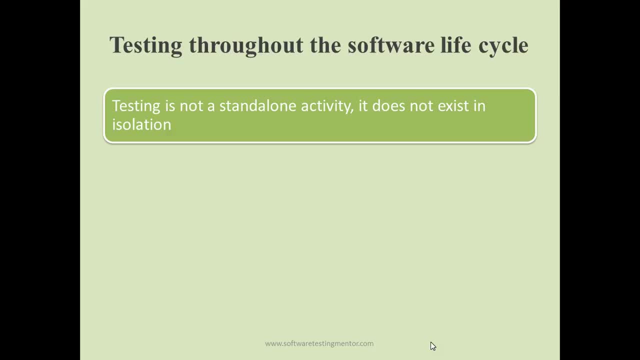 the development model. testing has its own place in the development methodology And it's not a standalone activity. It's present in every concept of blockchain software development, in every world of to have data all over the hospital line with us and the magic of the technology. that will provide that next step for the搜 incstrings. So one thing: I would richly like to thank everyone for communicative audience to participate in the webinar that we are doing. enjoyment today. I will wanted to thank everyone for your security visits. this video looks: 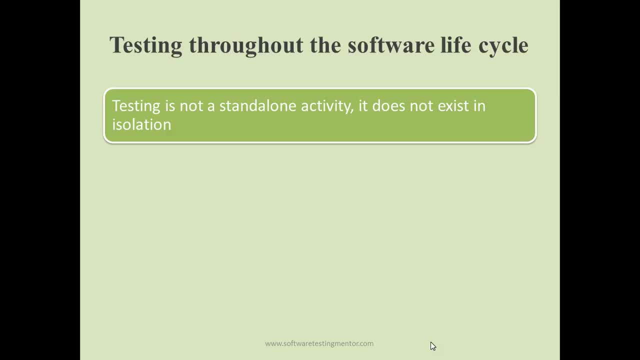 a great pleasure to the viewers. So today we'd want to breeze through the talk and take a過청 gam breach whole development life cycle. it's a life cycle activity and it does not exist in the isolation. so testing has its place in sdlc. depending on the development life cycle, testing has its place. 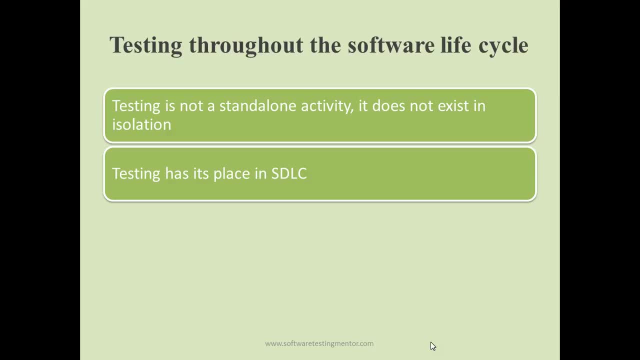 in the sdlc. if it's a waterfall model, if it's a v model or agile development methodology, testing has its place in every methodology. then the selection of software development model decides how testing will be organized in that methodology. so if you are selecting a waterfall development model for developing a software, the organization 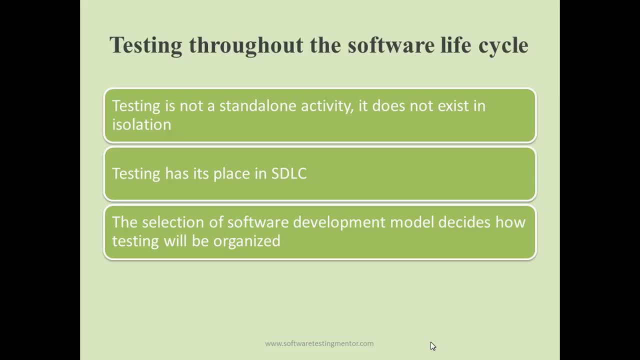 of testing in waterfall development methodology will be different than the organization of testing in V development model. so depending on the model, on the development model that you choose for developing, any software testing organization changes accordingly. so in V development model organization of testing will be different than the organization of testing in waterfall development. 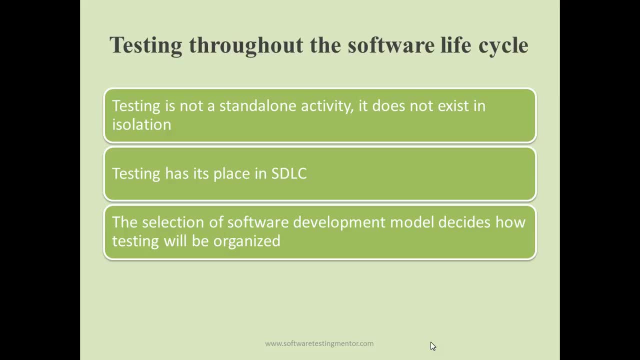 model. similarly in agile development methodology testing organization will be different. so the selection of software development model decides how testing will be organized within that development model. and there are different test levels in SDLC. so in software development life cycle there are different test levels. so the first test level you can say is unit testing. 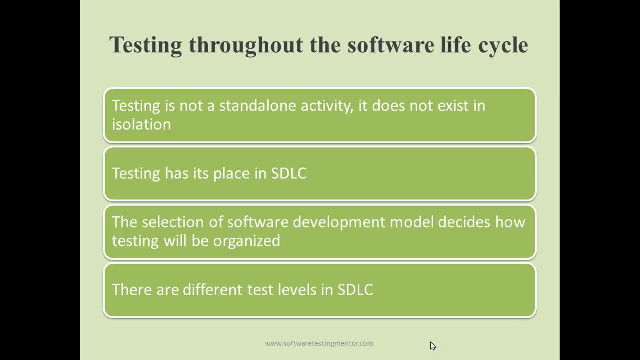 which is mostly done by the developers. so they write, they do the coding and then they write unit tests for the code that they have developed, whether those, you know, smaller chunks of smaller modules are working fine or not. okay, then you have integration testing, then you have system testing and then you have user. 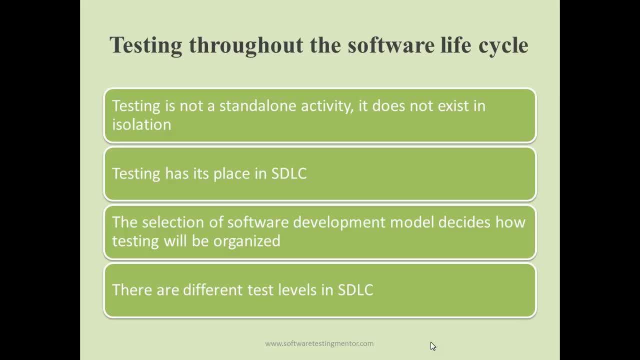 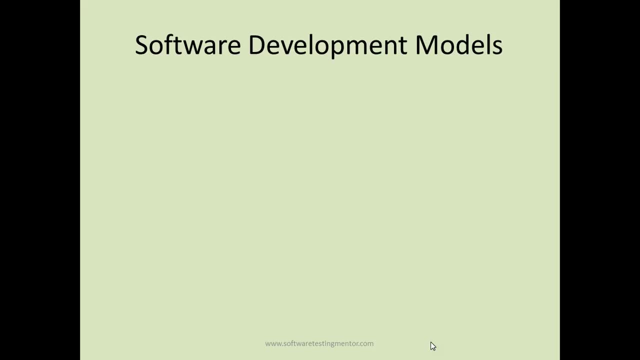 acceptance testing. so we'll we'll cover all these test levels in detail in further sessions. so there are different test levels in development life cycle then software development model. you can see that there are different test levels in development life cycle, then software development model. so there are different software development models. so the initial model is waterfall development. 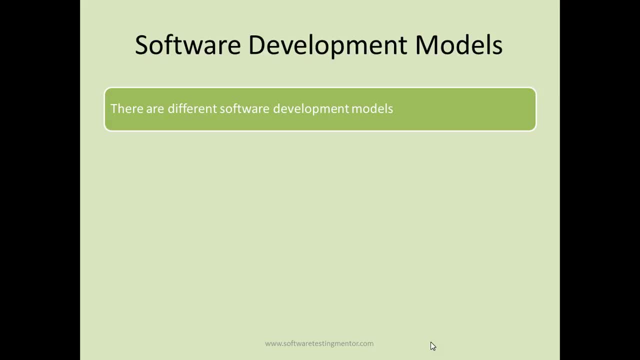 model. then, to overcome some shortcomings of waterfall development model, V development model came into picture which overcome some of the shortcomings of waterfall development model. then there there came in few more development models like iterative development model, which which have rapid application development and agile programming. Agile is the latest one nowadays. 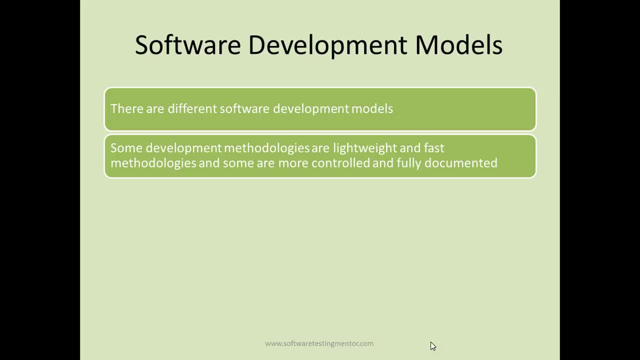 Then some development methodologies are lightweight and fast methodologies and some are more controlled and fully documented. So, as many of you would be knowing that the initial development methodology, like the waterfall development methodology, was very controlled and fully documented methodology. What this means is in waterfall development methodology, 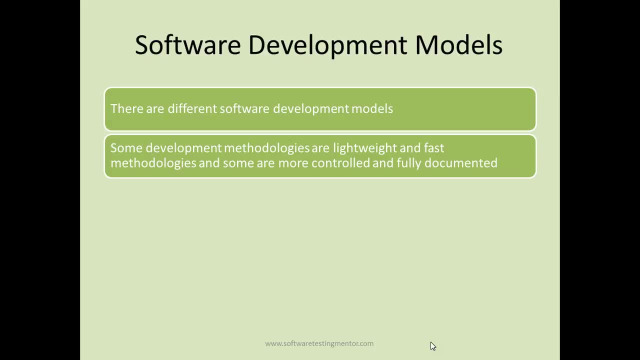 everything was completely documented, All the requirements were being finalized. Unless and until requirements were being finalized, you cannot go into the design phase. Once design has been fully documented and finalized and approved by all the stakeholders, then you go into low-level design. 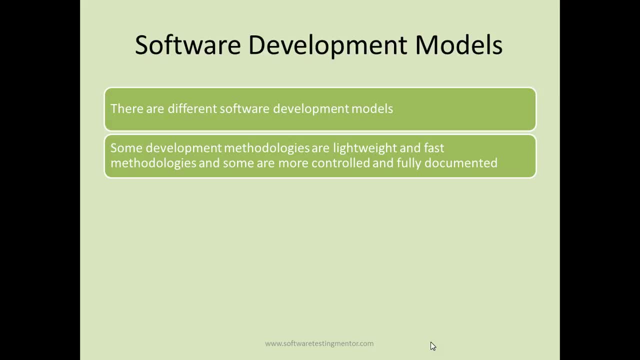 Once low-level design has been documented and approved, then coding started. Once coding is done, finished, only then testing starts. So waterfall development methodology was very controlled and fully documented methodology, But nowadays there are very lightweight and fast methodologies like agile. 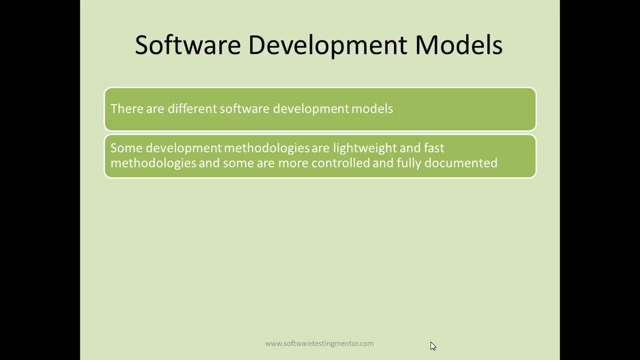 Agile development methodology is very fast and lightweight methodology because there is not much documentation involved. Agile development methodology is very fast and lightweight methodology because there is not much documentation involved. So very minimal documentation is done in agile methodology And there are sprints of two to four weeks cycle. 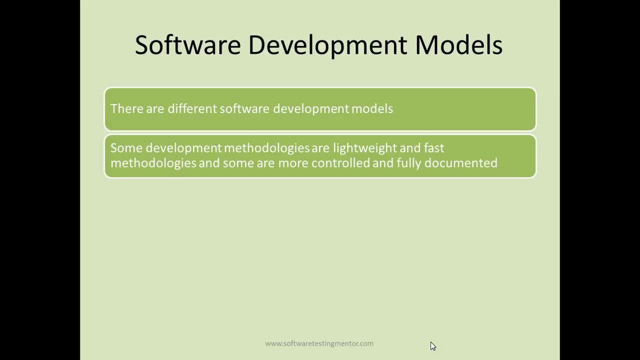 So in this timeframe of two to four weeks you have to design, develop, test and deliver, And after testing you need to showcase to the stakeholders whether the product that has been built in that sprint meets end-user requirements. So agile development methodology is very fast and lightweight methodology. 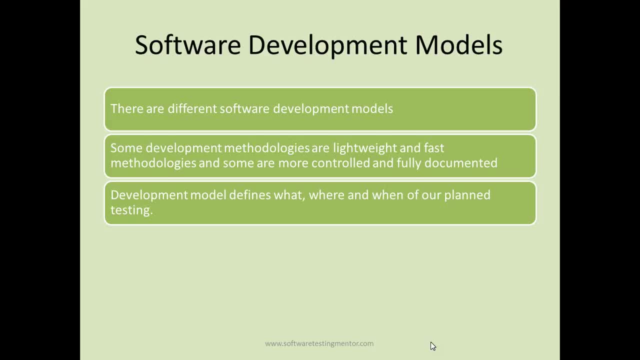 Then development model defines what, where and when of our planned testing. So, based on the development model that you choose, it defines how the testing will be planned in that development model, What you will test, where you will test and when will you test. 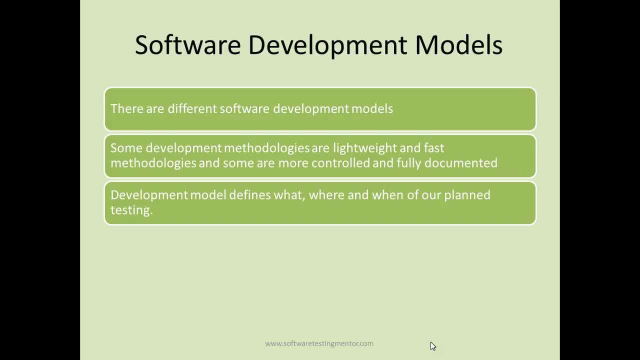 So if it is waterfall development model, your test planning for waterfall development model will be fully controlled and fully documented. For V development model it will be different. For agile methodology it will be different. So, based on the development model, test planning is defined. 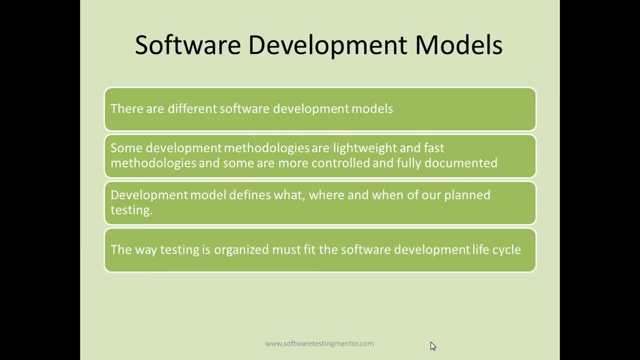 So based on the development model, test planning is defined. How the testing is organized must fit the software development life cycle. So your test organization, how you organize the testing, must fit software development life cycle. If you have chosen waterfall development methodology, your testing, the way that you organize your testing, 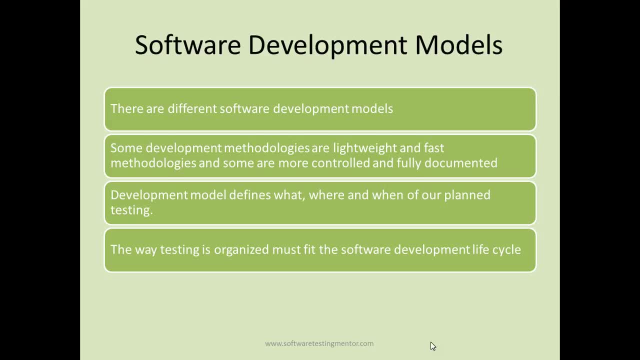 should fit waterfall development methodology. If you are following V development methodology, organization should should fit that V development methodology. so, based on based on the development lifecycle, your test, your test test organization should fit in every development lifecycle. verification, testing and validation testing is done so in based on different development methodologies. so whether 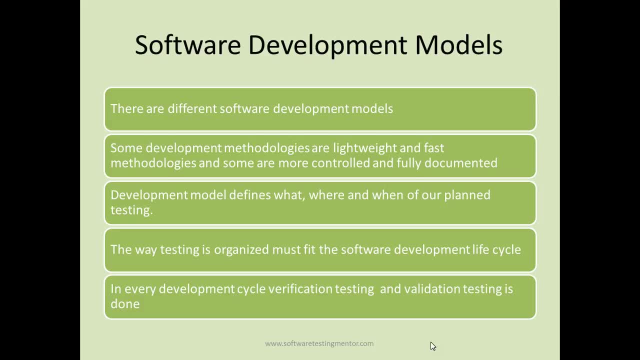 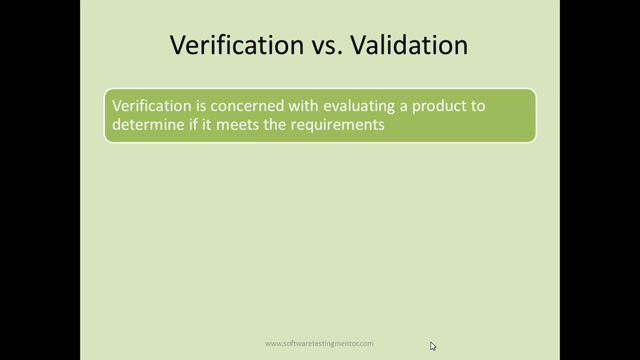 it is waterfall, whether it is V or it is agile, in every development lifecycle you do verification and validation testing. we'll cover difference between validation and verification in next slide. so verification is concerned with evaluating a product to determine if it meets the requirements. so verification is concerned just with the requirements. 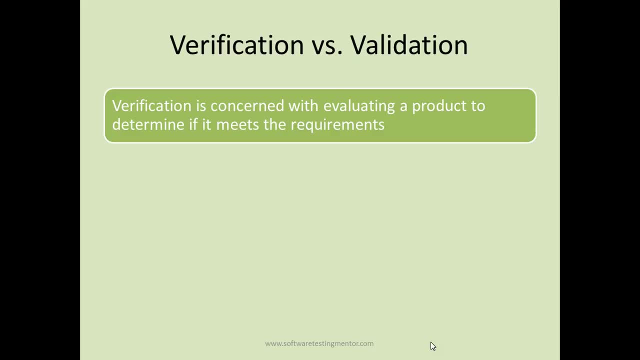 if you have the requirement, you have gathered software requirements in, you have approved software requirement specification document, the verification is just concerned with those requirements. if the software that you are testing is built as per the requirement, verification just checks that. so verification answers the question: is the deliverable build? 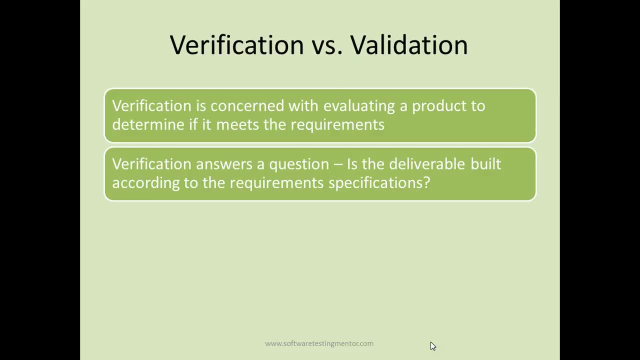 according to the requirements specification. if the deliverable is according to the requirements specification, that's fine, so that that part is taken care of by the verification testing validation, on the other hand, is concerned with evaluating a product to determine if it meets the end-user requirements or end-user needs. yeah, so there might be some. 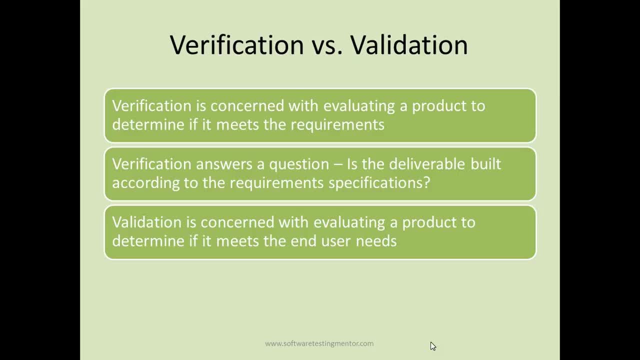 requirement which is not correctly captured and the software is built as per the requirement. so verification won't be able to find the defects, those kind of defects. so validation is concerned with evaluating the product as per end-user needs. validation answers the question: is the deliverable fit for purpose? okay, so validation checks whether the software that is being delivered is fit for. 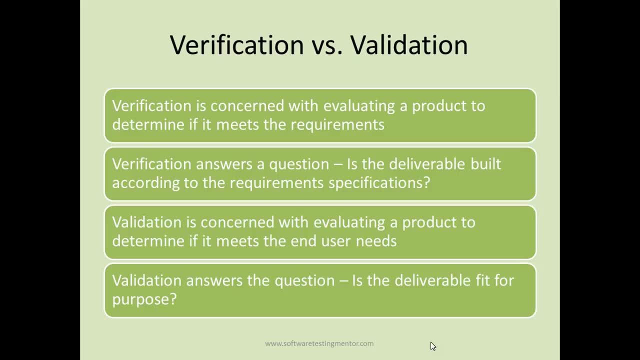 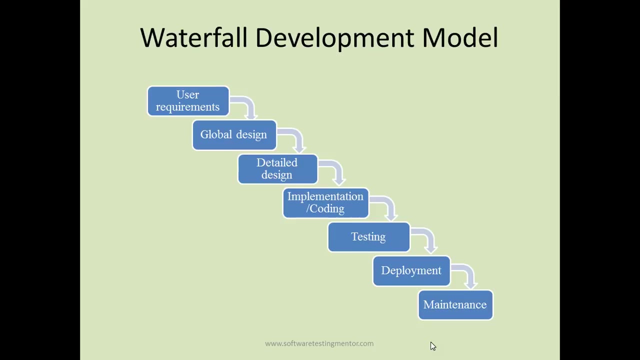 use or not, whether it's easy to use or not. okay, so validation is concerned, whether a deliverable is fit for purpose. now, the first uh development model is waterfall development model. so in waterfall development model, as you can see, it was, it was pretty straightforward, i mean you. 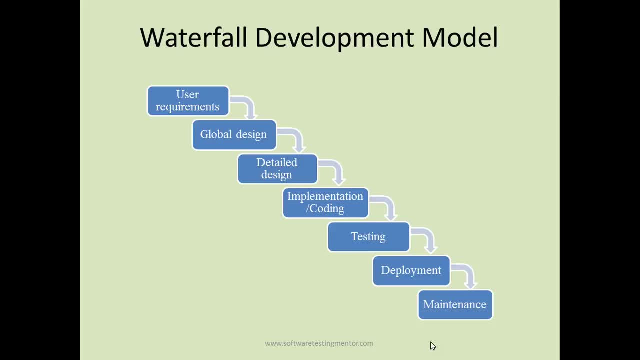 you have different phases in waterfall development model and you could enter into another phase only if first phase has been, you know, completely finished and approved by the stakeholders. so the first phase of waterfall development model was the user requirements phase, in which business analysts or product managers gather requirements from end user or from the the market, so depending. 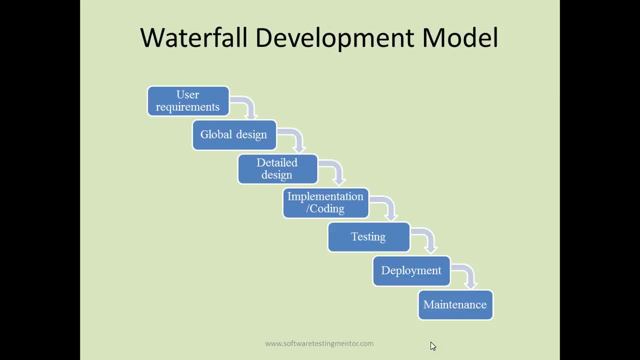 on the kind of software that you are developing. if you are developing a software for the client, you can gather the requirement from from the client. if it is a software being developed for a mass market, then you gather the requirement based on the already available products in the market. 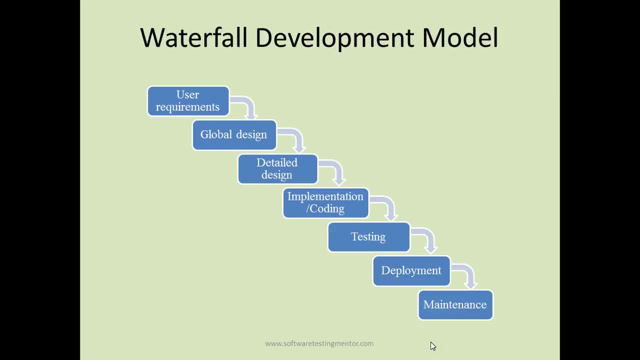 you evaluate them and gather the requirements. product managers gather requirement from competitors, from the actual end users that will be, you know, using those software. so in the user requirements phase, you gather those requirement, you capture everything, you create a document, software requirement specification document. once the document is created, it was sent for approval. 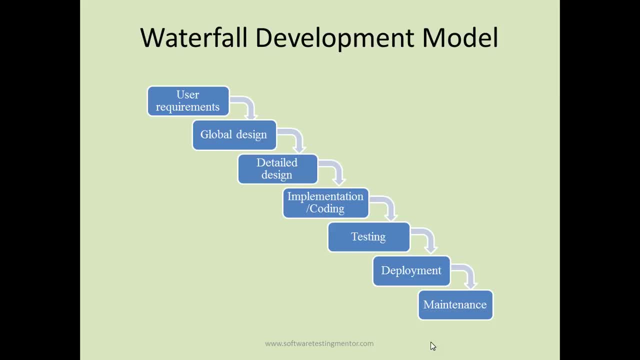 once all the requirements were approved, then you moved into the next phase, that is, the global design phase. so in this design phase all the high-level design was being done. so how the system will be, you know, built how, what, what database integration will happen, what database will be supported, what web server will be used will be supported to all those high-level design. 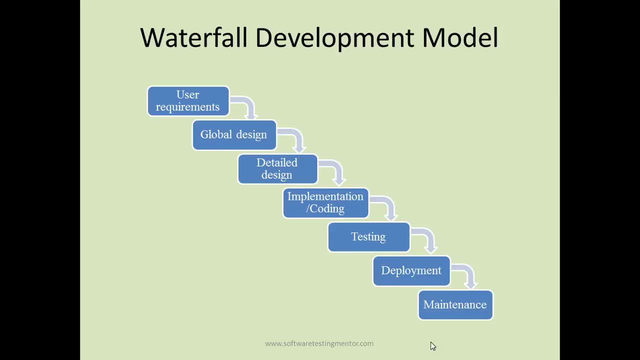 details were being captured into global design phase. so high-level design document was being is is being developed, sent to stakeholders. once design has been frozen, has been approved, then you move into the next phase, that is, the detailed design phase. so in detail design phase you develop low-level documentation, low-level design. 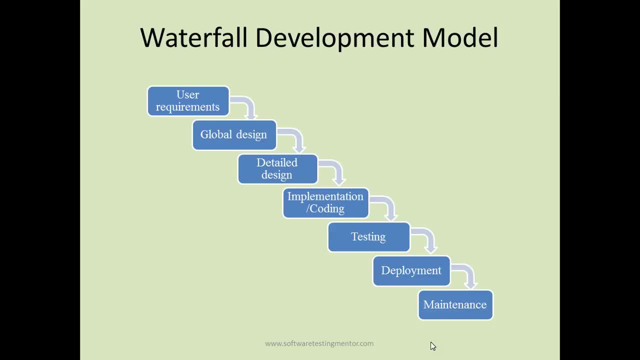 document which takes module different modules in greater detail, and how you design different modules of the software. what? what will be designed like for smaller chunks, smaller modules of the software? so then, after high-level design, low-level design was done and sent to all the stakeholders, product managers, technical architects- for review. so once that design has been completely, 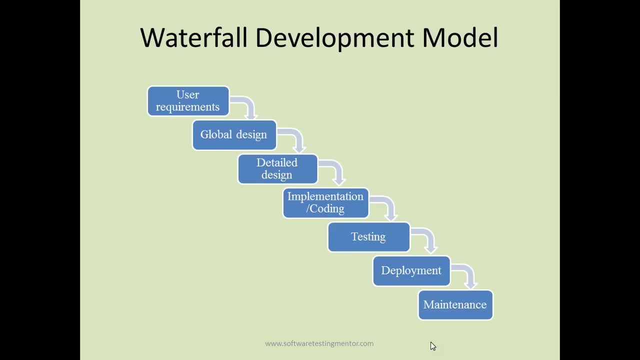 made, documented and approved. only then implementation or coding part started. so, as you can see in waterfall development model, you cannot move to next phase unless the previous phase or previous um step has been, you know, completely completed. um, it's complete, it's approved by the stakeholders. so, after the implementation, so after low-level design, 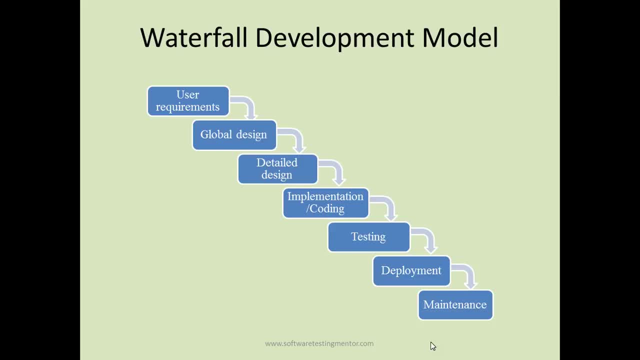 developers start coding implementation. they do some implementation. they, once the requirements are. some of the requirements are being bundled into the builds. builds are given to the testers which they install on the supported platforms and start testing. so after all the implementation has been done, testers start getting built. they, they start. 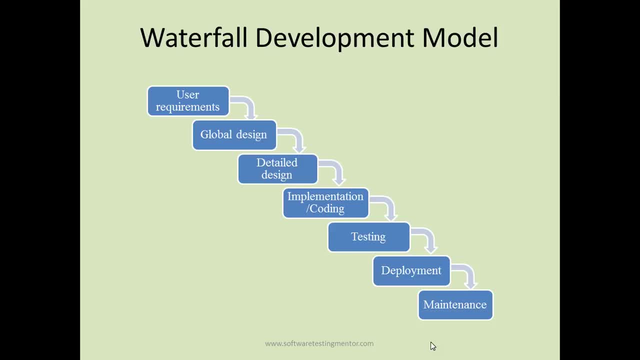 start testing. the raised effect developers raise the, raise the deep developers fix the defects and they keep on getting bills with new functionality, with defect pictures, and they keep on testing. so once testing is complete, all the severe, all the seven defects have been, you know, fixed and the 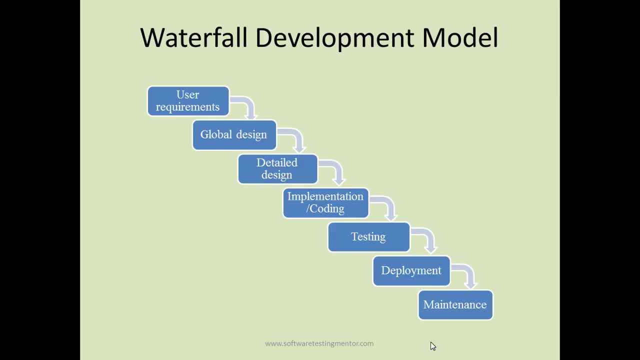 product or the software meets the exist criteria, it is being moved out of testing phase and is deployed. so after the deployment, after live deployment, then maintenance phase started for the software that is being deployed. so in in waterfall development model. it was pretty, I mean, was straightforward, but it was. there was no kind of unless and until you, you freeze the. 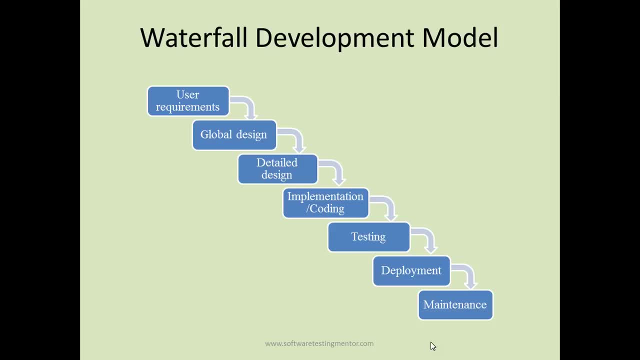 requirements. you cannot go to global design phase unless and you freeze the design, you cannot go to low level design. so that was kind of drawback in waterfall development model. but since this was the first development model you know in the industry so it was there for quite a long time. so to overcome the issues that were there in 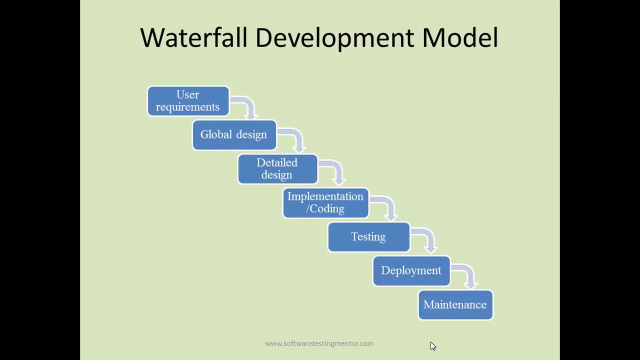 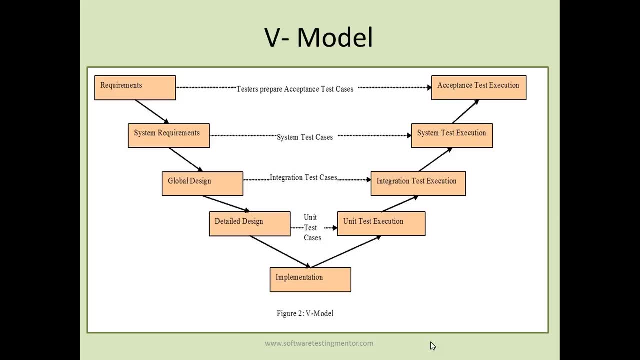 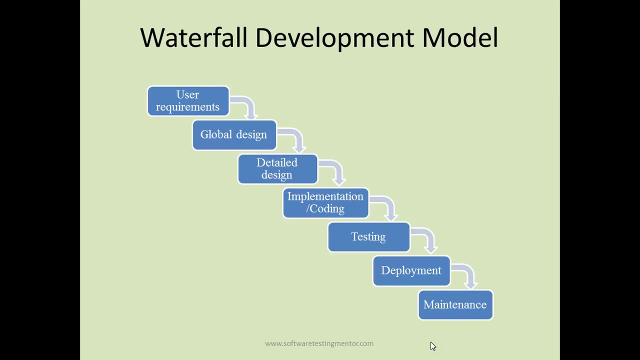 waterfall development model. another model came in that is known as V development model. so in V development model, if you see, testers were involved right from the beginning. so if you see the waterfall development model, testing came after four phases were done. so what if there were issues in the requirements? what if requirements were not being captured properly and are not testable? 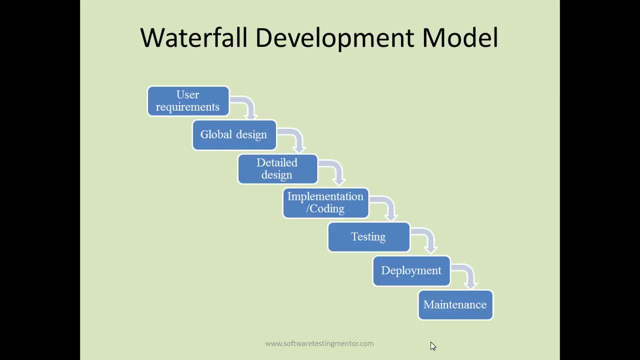 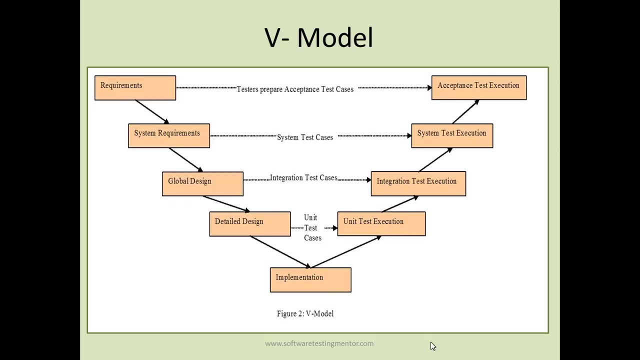 so testers never knew if the requirements are not even you know if the design is not proper. so, to overcome all these issues, because since the feedback from test team was not not there in waterfall development methodology, so we model came in wherein testers were involved in all phases of development lifecycle. because of all those issues in 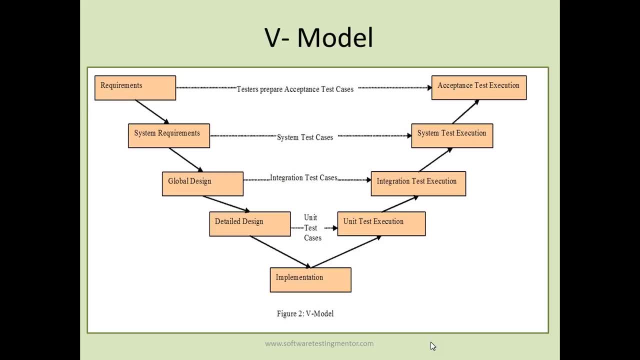 waterfall development methodology. there were a lot of issues, so suppose there was a requirement issue and requirement was not being. requirement itself is not valid, so that used to be detected when testers start testing and the organization has already already invested money in requirements gathering, in designing and developing. 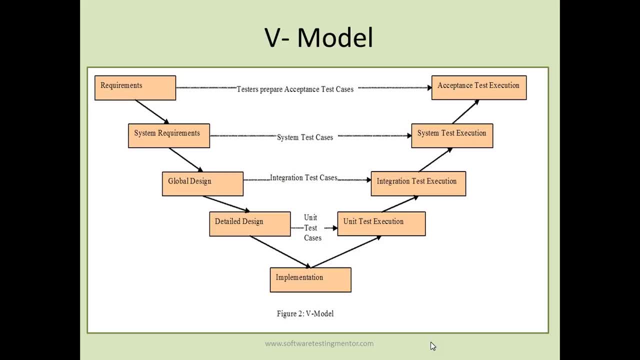 and then the testers found that there the requirement itself is not valid or the design there is. there there are design flaws, um in in in the software. so at that point of time the cost of again capturing correct requirement or redesigning is very high. if, um, if it would have been, you know, 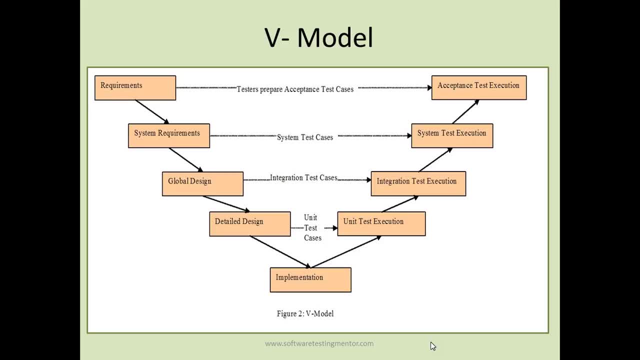 um detected well in advance. so in v model testers are involved in all the phases. so right from the requirements testers in in the requirements phase testers prepare acceptance test cases. so when the requirements are being gathered they validate those requirements and they prepare acceptance test scenarios in in that phase. then in the next phase in the system requirements, when 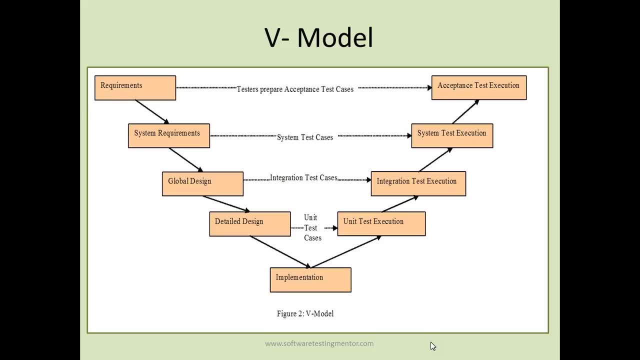 system requirements are being gathered, whether the which database will be used or whether the lake test case, markup 말�u test case requires the 산 existed for the google software start preparing according to Accepted test case, because when the requirement is stopped and the program automation starts, they will start UPSTART when the model lock is turned ON. 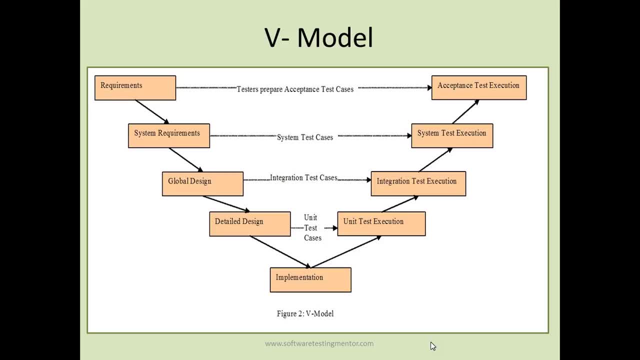 and when the gonna be doesn't allow the Ronald be launched, basing out to 0 in the app and start preparing and testing test cases for the Imran application. ти testing test case. understand how the, the design of the whole software will look like. testers prepare system test cases in in that phase they review the high level design, low level design and system requirements on global design phase and prepare system tests cases and into integration test cases. so in Global Design. 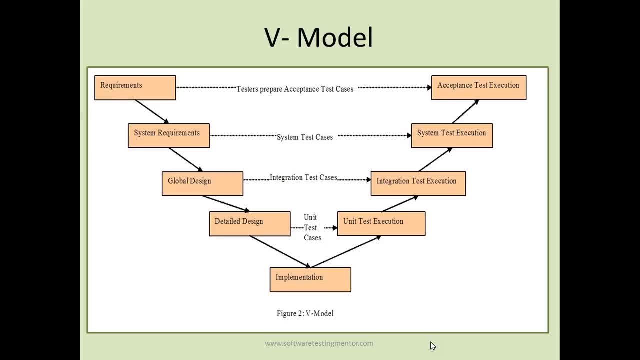 when developers or technical architect design do gameplay開心, exhibition design and tests cases and in integration test cases. so in global design, when developers or technical architect design- I'm- do a high level design, then testers create integration test case. so they go through the high level design thoroughly and create integration test cases and also validate whether the design is. 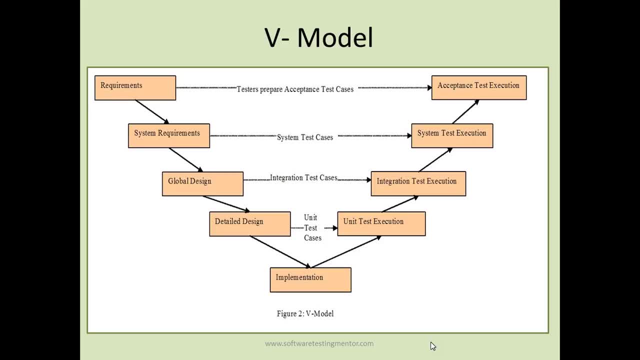 is proper or not. then in detail design testers create. it's mostly a developer's activity in detailed design most, most in most of the organization you'll find that unit testing is done by developers. but yes, testers do provide input in unit test cases as well. so in detailed, 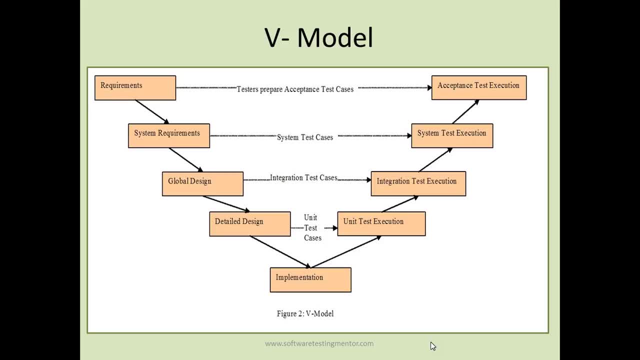 design phase, testers provide input in unit test cases and then, after detailed design, implementation is done and then testers start once the implementation is done, testers get the bill after the unit test is done. so it depends. so there are organizations wherein unit testing is done by testers as well. but 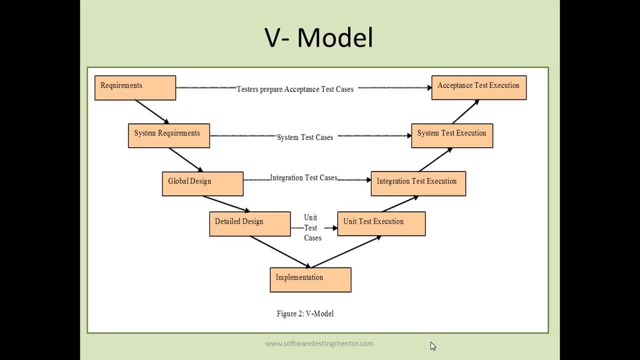 at most of the places you will find, unit testing is done by developers. it's very rare that unit testing will be done by testers, so developers will implement the code, they will do the unit testing and then testers will start integration test execution. they will start integration test cases. 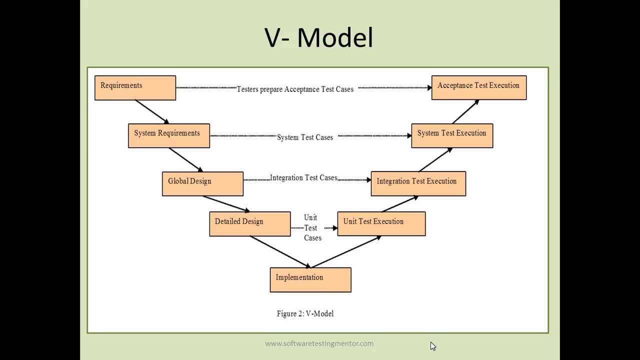 once integration test test is being done, then they'll start system test cases and then once system testing is done, they'll start the acceptance test test cases. so v model overcome all those issues that were present in waterfall development model. so in v model if there is any issue with the requirements itself, requirement is not valid, it is not captured. 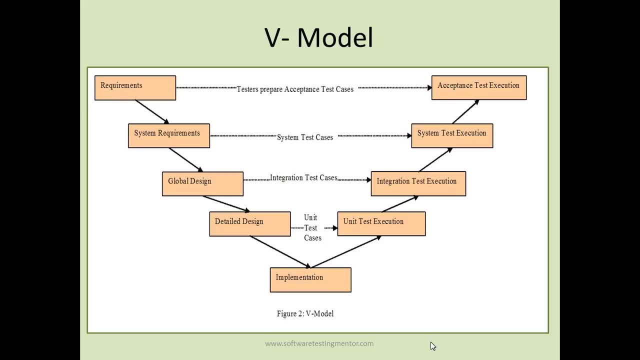 properly. testers will point out that well in advanced if there is an issue with system requirement or if there is an issue with design. so testers review all those documents and they they provide feedback then and there, and which avoids a lot of rework and a lot of savings. 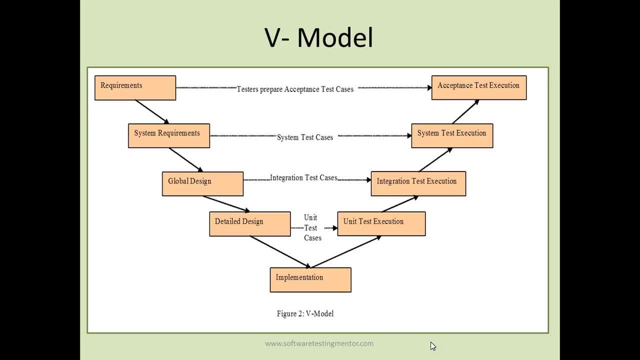 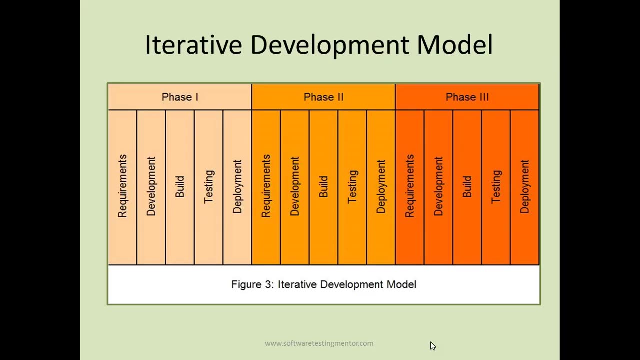 for for the development. but in waterfall model there was no feedback being provided to the previous phases and because of that if there was any design flaw or requirement issue it took a lot, a lot of time and money to fix that. then the other software development model is iterative development model. so in iterative 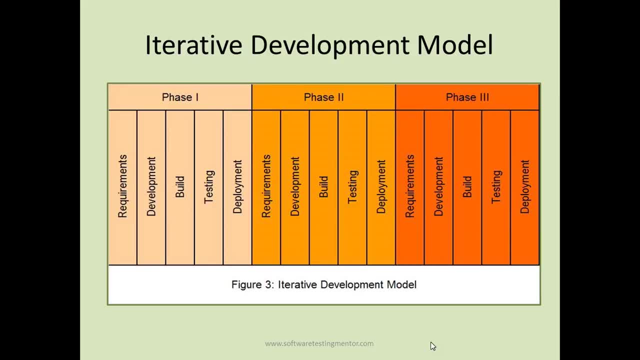 development model. usually you have um, a time boxed iteration, say two to four weeks. so depending, i mean that there can be um. if it is agile methodology, it will be two to four weeks um and there are some iterative development methodologies wherein you you use more than four weeks as well. so there are different phases um in iterative development model wherein you 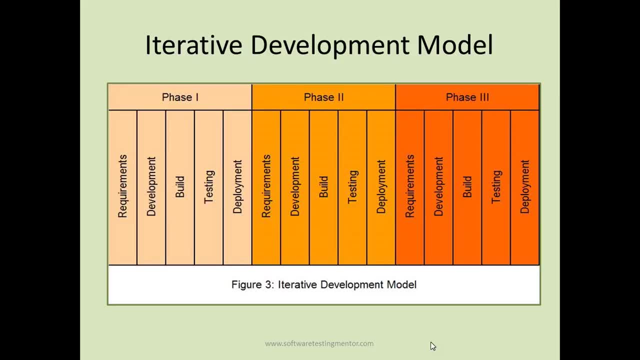 capture the requirement, you develop, you build, test and deploy. so, like you can see in the figure, in phase one you have, you capture requirement, you develop, build, test and deploy. and then in phase two, on top of whatever you have built, tested and deployed, you again capture new requirements, you develop them, build them, test. 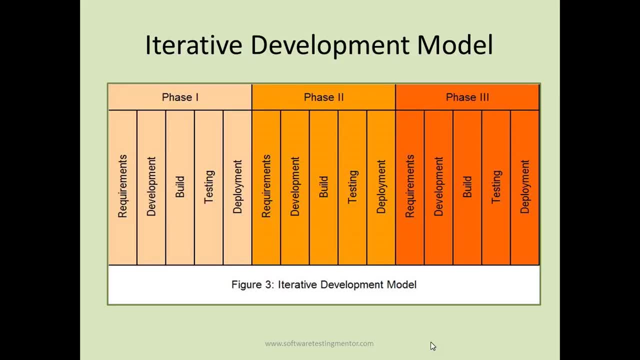 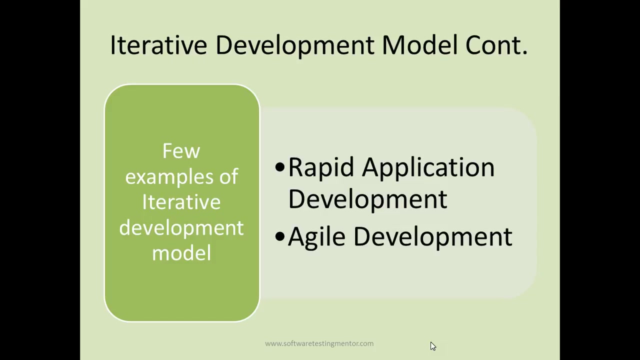 them and again deploy them. all right, so that's how iterative development methodology is done. so you have time box iterations and you do all your your development activities in those time box iterations. so iterative development model- uh, some some of the examples of iterative development model are rapid application development and agile development. so rapid application development is. 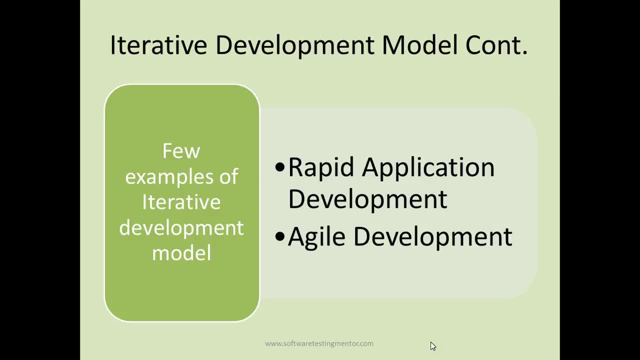 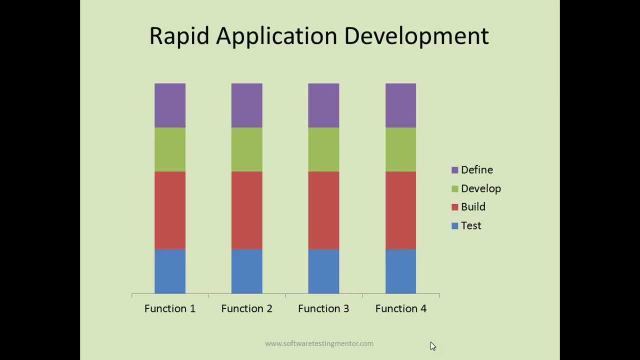 also a development methodology, which, which is iterative development methodology, let's yeah, so rapid application development in. in this methodology, you, you develop all the functionality at once, to suppose you want to build something. so there are, say, four functionalities being developed in an application to develop, you, you define you. 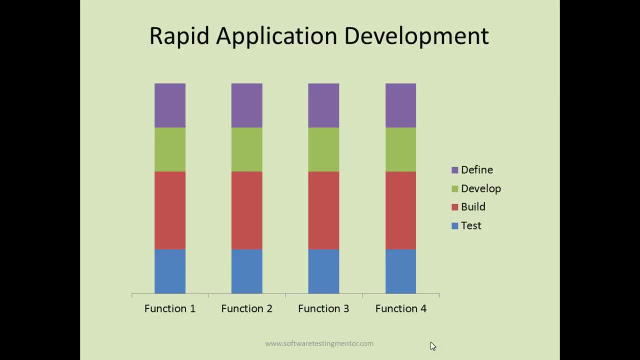 know some teams, small teams, and everything is built at once. so one one team will build function one. another team will build function to. 13 will build function 3, 14 will build function 4. so then what they will do is they'll define, they'll develop, and then define, develop, build and test. so 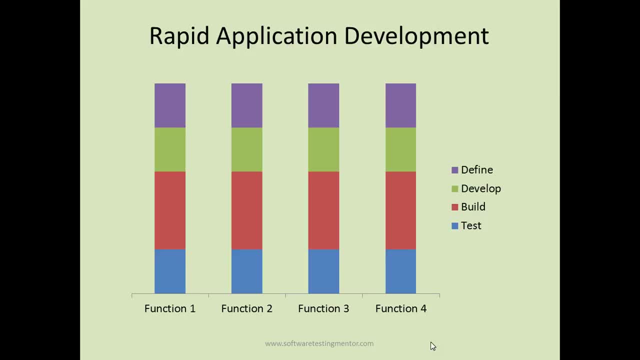 these teams will do all the development functionality, or that all they'll. they will gather, the they'll design, defined, their develop, they will build and they will test all the different functionalities and then all these functions are integrated into one and then a working product is being demoed to the stakeholders. 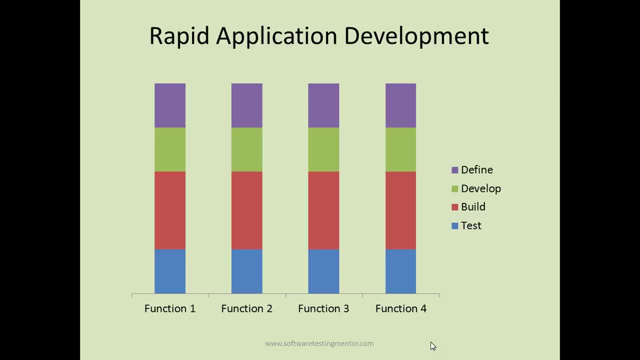 so this rapid application development is quick and easy. a quick, quick methodology just to give a rapid feedback to the stakeholders so that they are aware how the system looks like, rather than spending months of effort in gathering, requirement, design, develop, test and then at the end of a year. 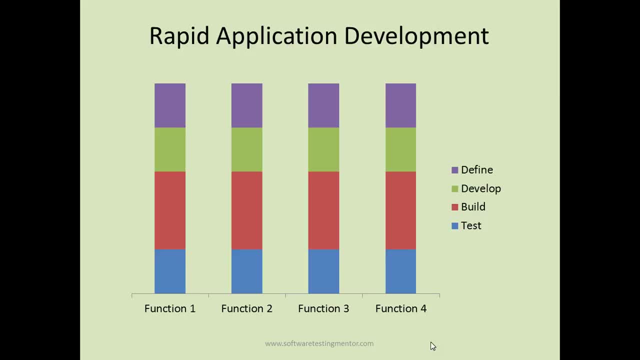 knowing that no, this is not what we wanted. so they this rapid application development approach is is quite easier and it takes less time and effort and and budget. so every function is being implemented all at once and integrated with Big Bang methodology, integration methodology and demoed or showcased to the stakeholder, and then the the stakeholders decide whether to continue with with. 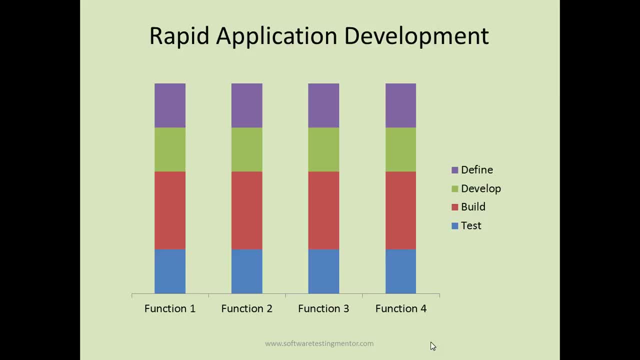 the application that has been developed, whether it has been built as per requirement or whether it will be. you know kind of whether it makes sense to continue with it or whether to discard it and start with some other idea, or start with some other modifications and then go ahead. 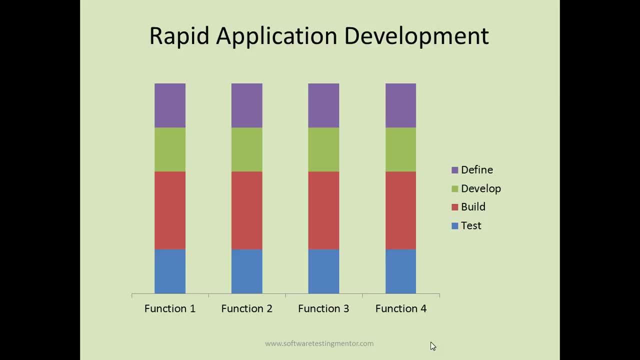 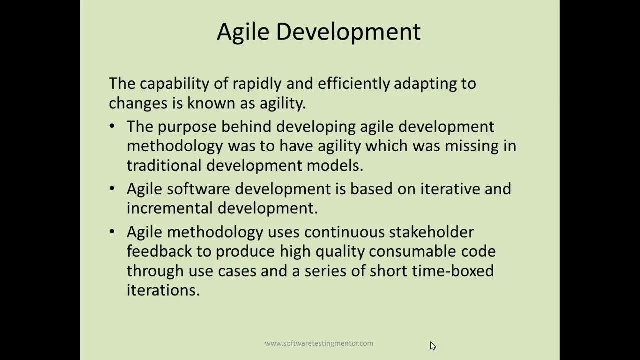 with the development, so it gives very early feedback to the stakeholders and saves a lot of time and money for the organizations. then you have Agile development methodology. so agility is something to capability of rapidly and efficiently adapting to changes. so Agile came from the word agility and Agile is capable of rapidly and efficiently adapting to changes. so that's where Agile 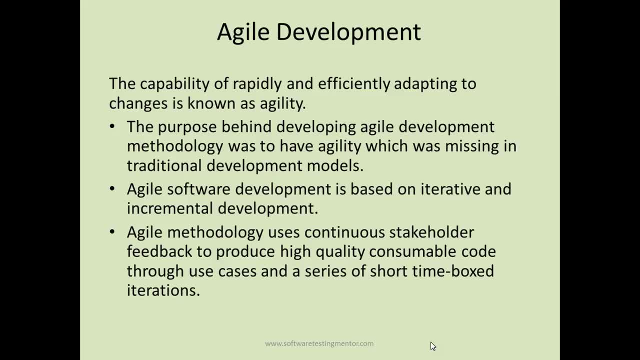 development methodology came from. so the reason behind developing Agile methodology was to have agility, which was missing in traditional development models. so if you consider waterfall development model or V development model, so there was very, very less chances of less agility there because requirements has to be finalized, design has to be finalized. only then coding starts, then testing. so it was kind of very rigid approach. 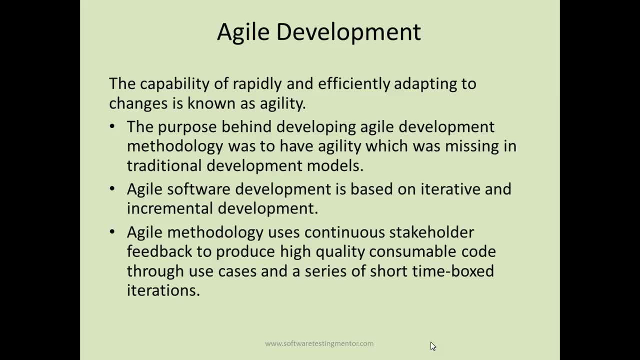 towards developing the software and that was not good, because if a stakeholder came in and he he saw the software and he thought of no, I don't like that and I want to get this change, then he has to again. I mean, every process has to follow again. you need new requirements being captured, design, development, all all that. 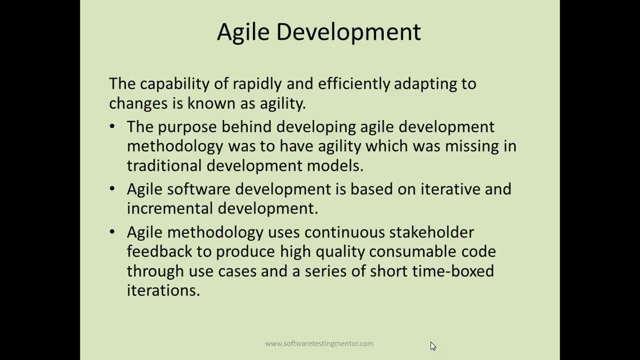 full flow. full development flow has to follow again. so that was that was the drawback in all those previous models: beat waterfall or beat V development methodology. so agile development has a development methodology, has agility to rapidly and efficiently adapt to any changes or any feedbacks provided by the stakeholders. 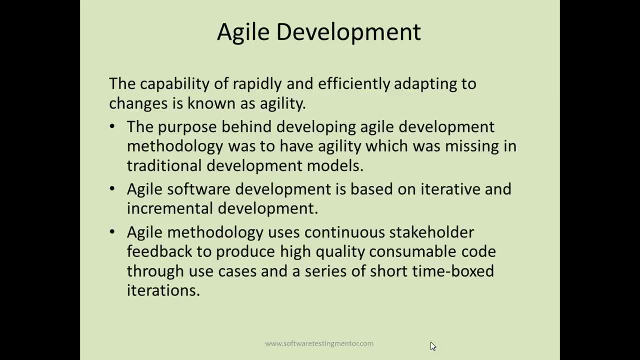 so agile development development is based on iterative, incremental development. okay so so agile is a part of iterative development methodologies. agile is agile development methodology is a two to four weeks cycle, so depending on on different organizations they choose, some organization choose two weeks sprint, or some organizations choose. 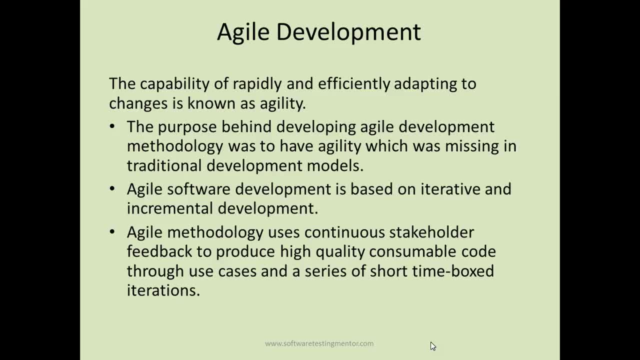 three weeks. some also choose four weeks sprints. so based on how, how the organization wanted, they choose those prints and then all the requirements are being gathered at once and lie into the product backlog. once everything is there in product backlog, then these prints start and those requirements or user. 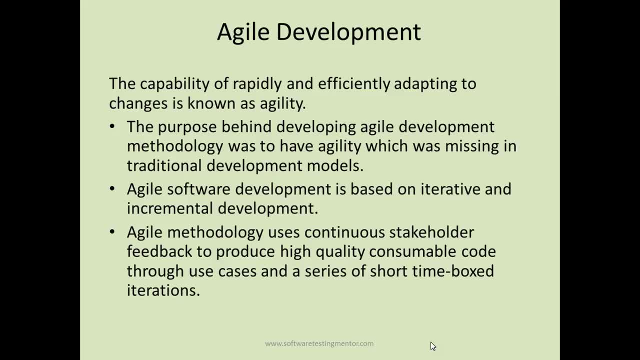 stories are being pulled from product backlog to sprint backlog and then sprint. there are scrum teams which take all those requirements based based on different scrum team or different modules. the scrum teams are being organized so they take the requirements and the design, develop, test and deliver a working product and 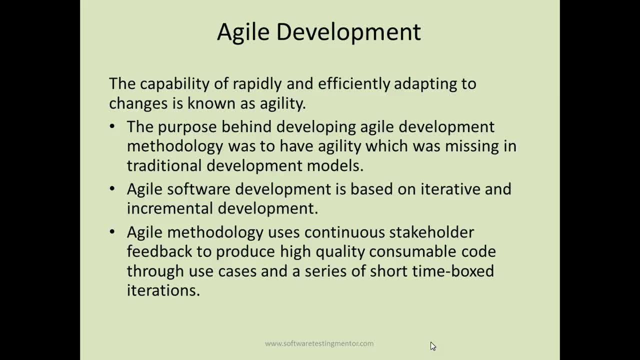 showcase a working product to the stakeholders after two weeks or three weeks of sprint and then, after showcase the, the feedback from stakeholders was taken whether things were all right, whether they want some changes or something is not right, if something needs to be changed. all those feedbacks were taken and then again in next. 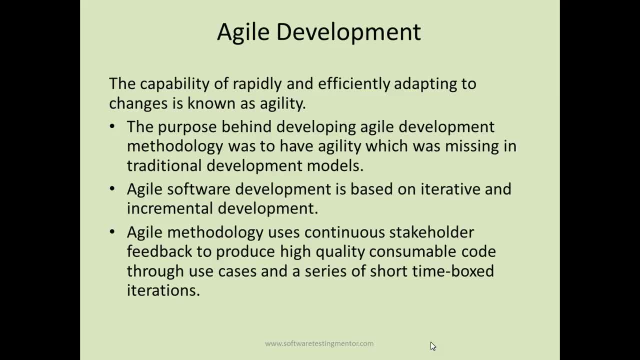 next sprint, those changes can be no taken care. so agile methodology uses continuous stakeholder feedback to provide high quality consumable code through use cases and a series of time box iterations. so these time box iterations are known as sprints, and in these sprints you pull the use cases or user stories from the product backlog into the sprint backlog and then you 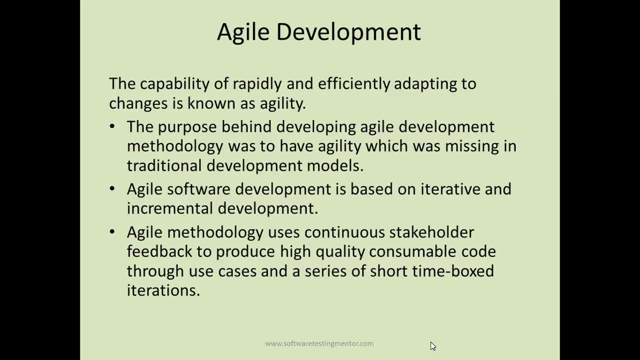 can use the user stories, to implement these user stories into a working product and then showcase these stories. at the end of this sprint and within these sprint, all the activity- your design, develop and testing activity- takes place. so after testing, any defect raise is fixed by the developers and 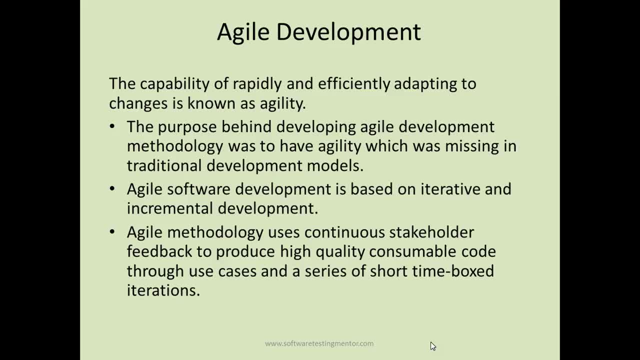 again retested, and once everything is tested and there are no critical defects, it is showcased at the end of the sprint for the entire sprint cycle. so in the next sprint the user stories are being taken and the端 data is being translated from there so that you can read the data and then 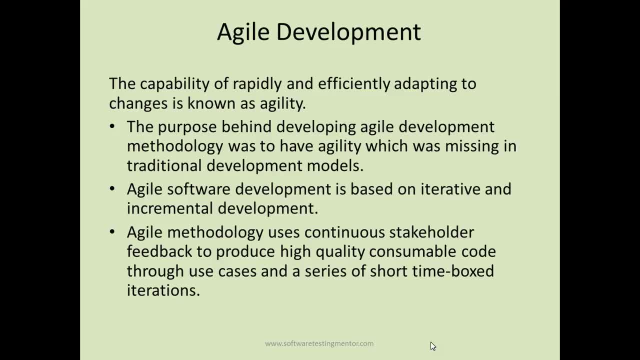 the pdf data will repeat itself for the next 2005 products and then on the next sprint. you will also see that in the next sprint, the user stories are also being asked and the user stories are being taken and the user stories are being implemented, and so this is the way that we 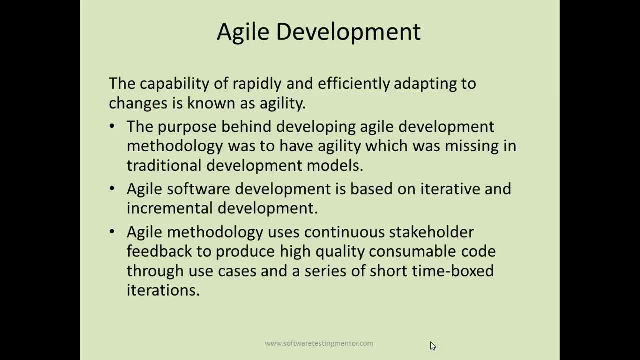 do it. so in the next sprint we will look at what we are talking about and then we will look at the once strats and then we will look at the following step-by-steps to make sure that the user stories are: the product is developed. the product is being developed with continuous 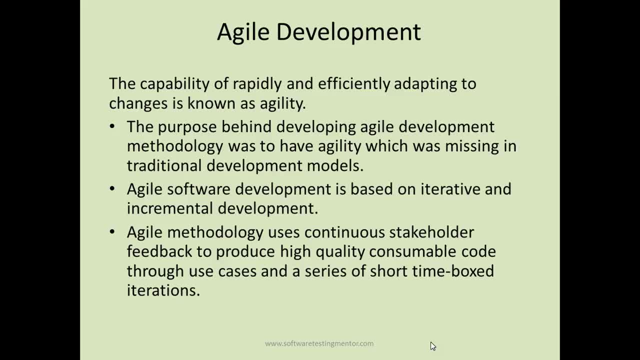 stakeholder feedback. so in agile development, whatever requirements have been being implemented in the first phase needs to be, you know, regressed in the second sprint, and whatever requirement have been implemented in sprint 2 need to be regressed in sprint 3, so so you can see, like in agile.